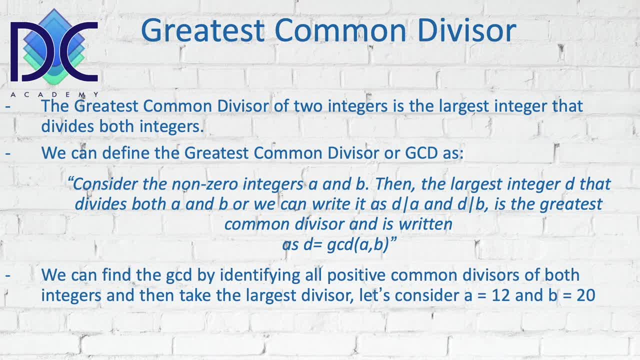 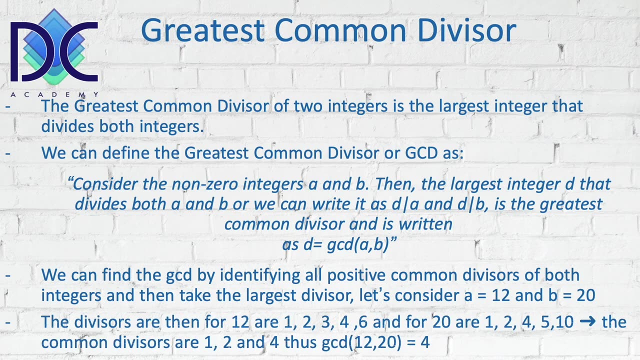 how to find it. Now, what we can do is to look at the positive common dividers of the two integers that we are considering. So we're just looking at, for example, at the numbers 12 and 12.. And you can find, or you can say, that the divisor for 12, for a are 1, 2, 3, 4 and 6.. 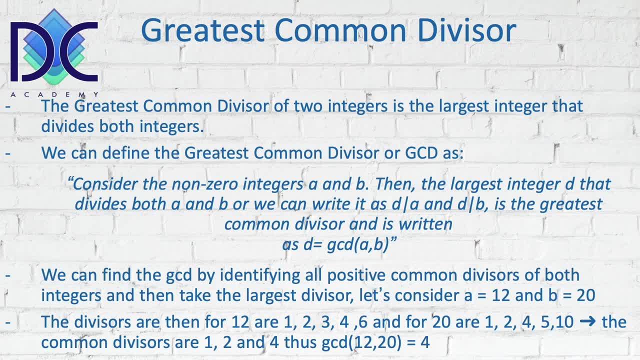 For 20, we have 1, 2, 4, 5 and 10.. And we see that we have common divisors here, which are 1, 2 and 4, and we say that the GCD is in fact of 12 and 4, sorry, 12 and 20 is. 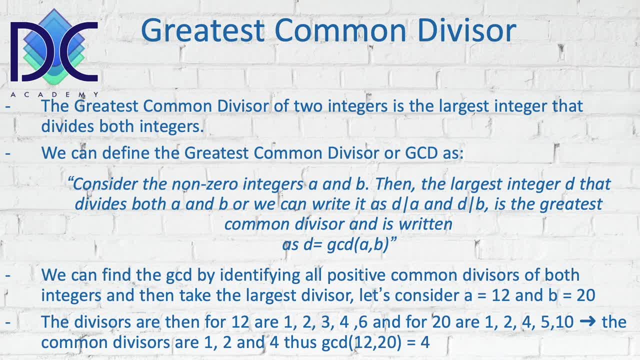 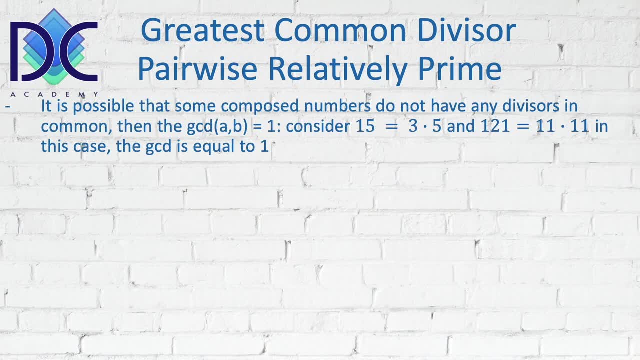 equal to 4.. So that's the greatest common divisor That we have in those two numbers. Now we look at the greatest common divisor and what we also call pairwise, relatively prime, When we have the greatest common divisor, and that greatest common divisor is 1.. So we can have composed numbers. 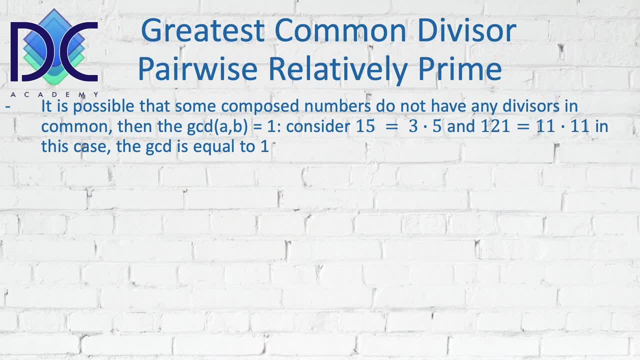 which are not prime numbers, that do not have any divisors in common, And when they don't have any divisors in common, we can say that the GCD, the greatest common divisor of those two numbers, is equal to 1.. Let's consider two numbers: 15, which we can write as 3 times 5, and 121, which we can write: 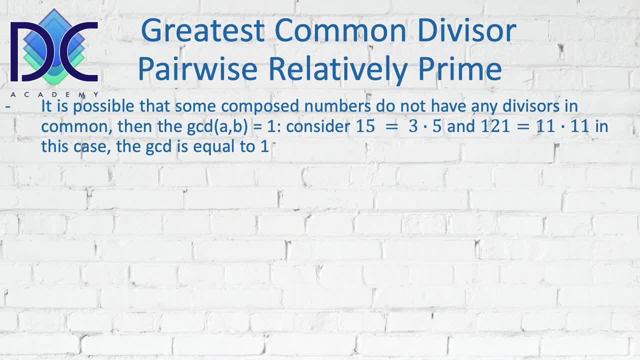 as 11 times 11.. In this case, because there are no common divisors, The greatest common divisor of those two numbers of 15 and 121 is equal to 1.. And then the greatest common to one. now, when two numbers have as greatest common divisor the number one, then we call them. 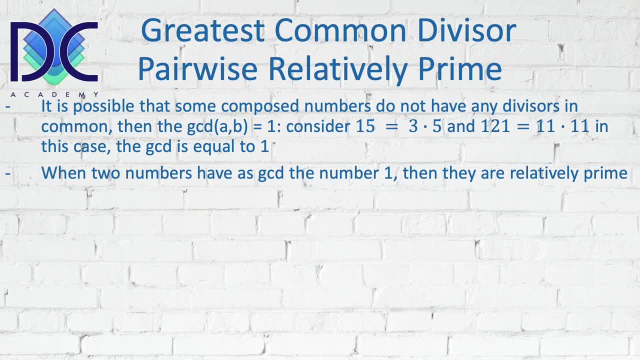 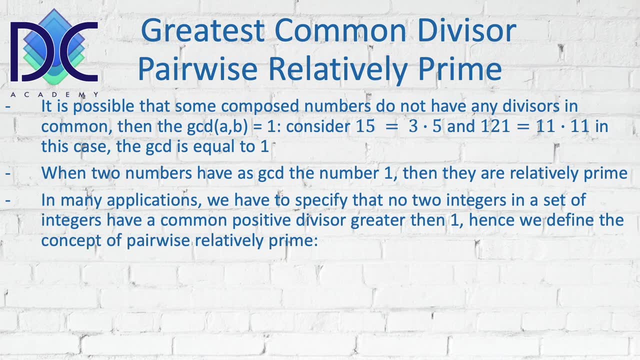 relatively prime, because they don't have any of those numbers in common. we cannot divide it by them. they're not prime number but they're relatively prime. now, when we have applications and we find in fact in a set of, let's say of when we have two integers in a set of integers, we try to 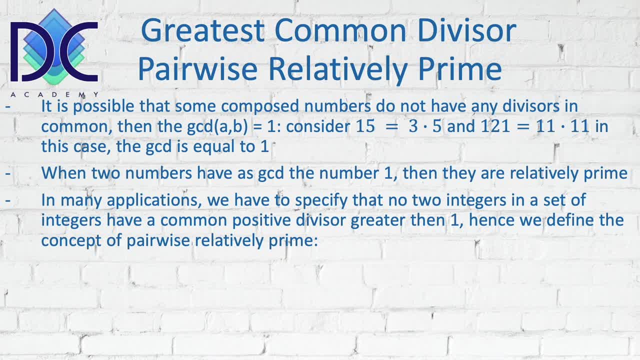 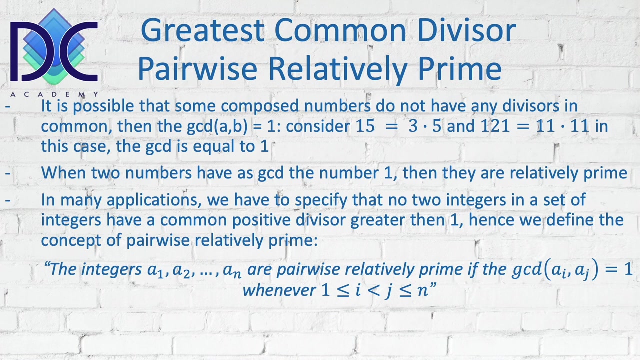 find those, those integers that have a common positive divisor greater than one. so it's basically important to define the concept of pairwise relatively prime. so when we have the integers a1 up to an, there are pairwise relatively prime prime if the gcd is equal to one of the numbers a i and a j, and that's whenever. 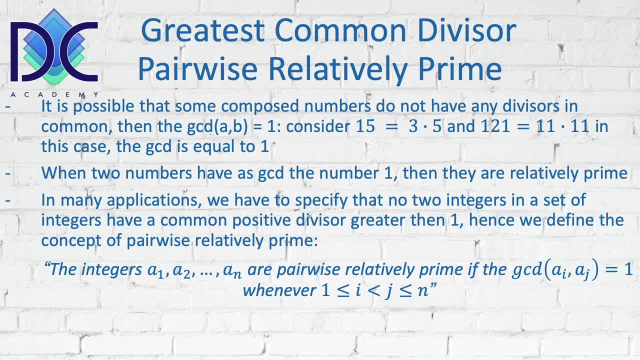 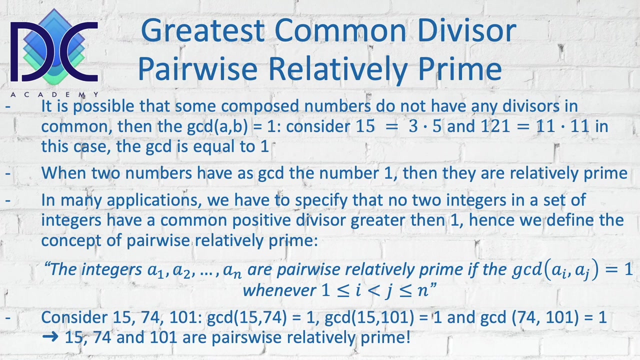 one, or i and j are between one and n, and j is larger than n. so we take different numbers, we take different integers and we try to find those integers which have a gcd equal to one. so basically, that's the concept of pairwise relative. we can say that the gcd of 15 and 74 is 1. they don't have any divisor in common, the gcd of 15 and. 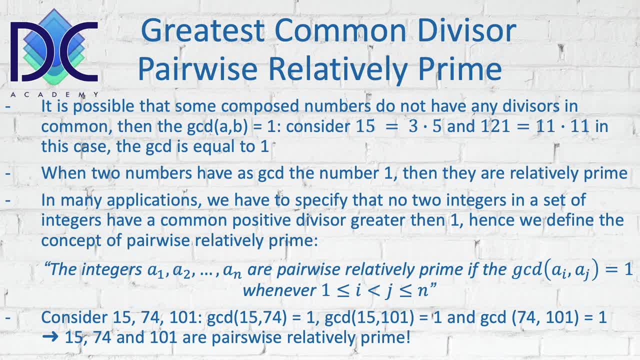 101 is also equal to one and the gcd of 74 and 101 is also one. it means that 15 is less than one to ум. 74 and 101 are pairwise relatively prime. So it's a very important element to understand. We will. 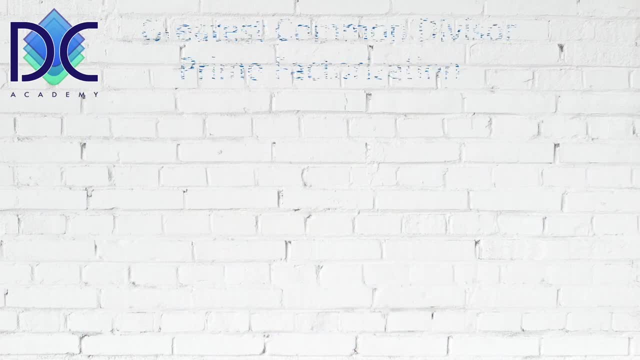 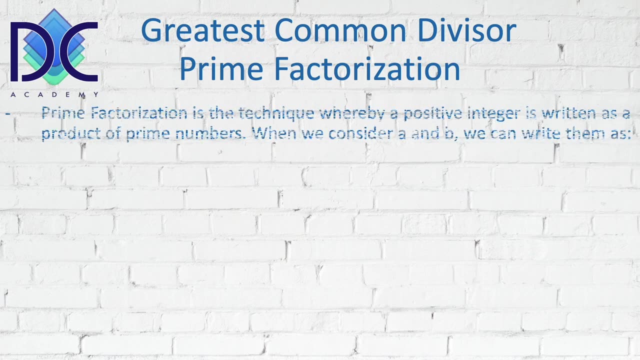 use it later in some applications. Now we are going to use the greatest common divisor and apply it to prime factorization. Prime factorization is a technique whereby a positive integer is written as a product of prime numbers. When we look at two prime, sorry, when we look at. 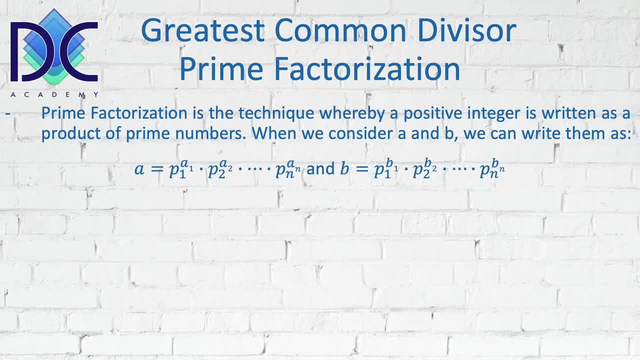 two integers, a and b. we can write them as: a is equal to the first prime to the power a1, multiplied with the second prime to the power a2, and so on, up till we reach all the primes that are relevant and their relative powers. We can do the same for b and we can say that some 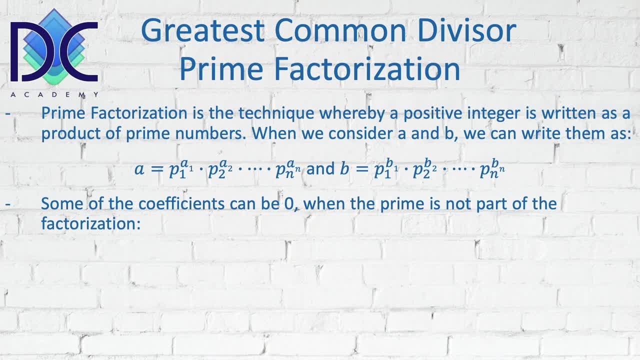 of the prime numbers are prime numbers, So we can write them as: a is equal to the first prime, to the power of those parameters, powers in this case a, i or b. i can be zero when the prime number is not part of the factorization. So let's have a look how we do this when we have two numbers. 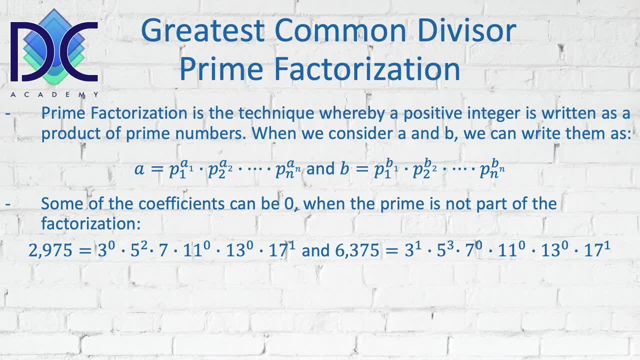 We have the number 2975, which we can write as a prime factorization. I didn't put there the first prime two, but we could put there two to the power zero, Which doesn't really have a sense here. but I put here the prime numbers that are common in the 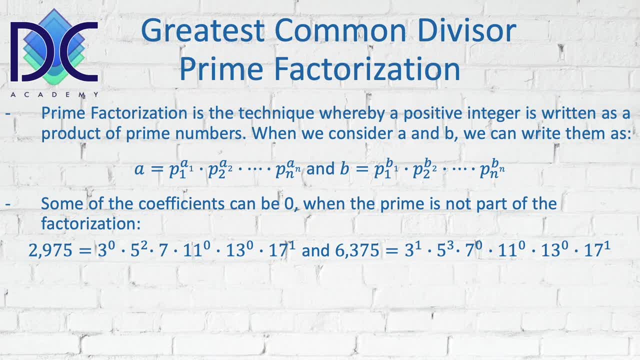 two numbers. So the first one I write here is three to the power zero, because 2975 cannot be devised by three, but it can be divided by 25, by seven and by 17.. So I have the factorization: three to the power zero times five to the power two times seven. 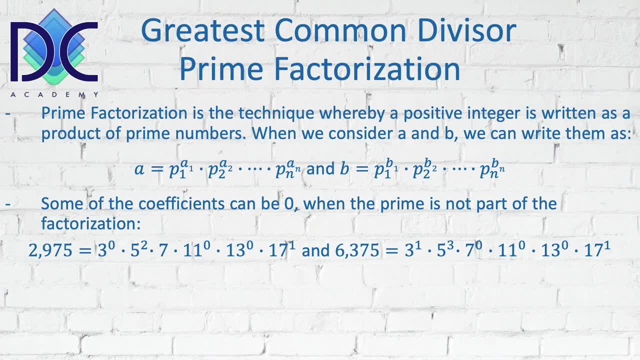 Times 11 to the power zero, times 13 to the power zero and times 17 to the power one. I could have left out those primes which have a power equal to zero, but I just leave them here. So you see all the primes that I'm considering and that some of those powers are indeed equal to zero. 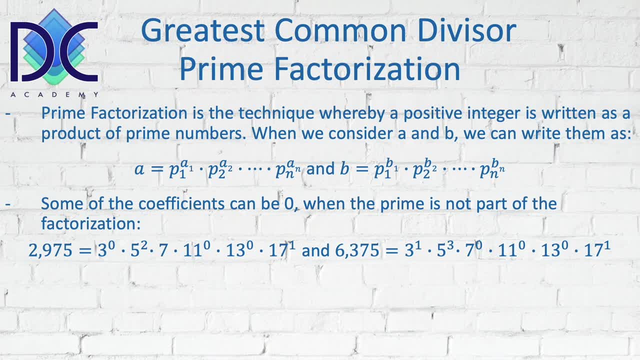 The second number that I have is 6,375, which can write as three times five to the power zero. So the first one I write here is three to the power three plus seven to the power zero, 11 to the power zero, 13 to the power zero and 17 to the power one. 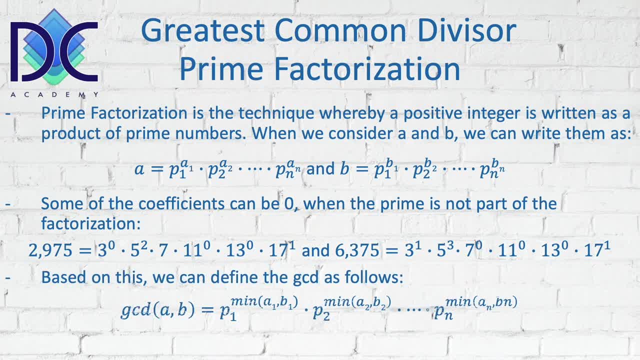 Now, based on this, what we also have is that we can define the greatest common divisor of two numbers as the product of the primes and the powers. But when I have the different primes, I take the minimum of the powers of the two numbers. 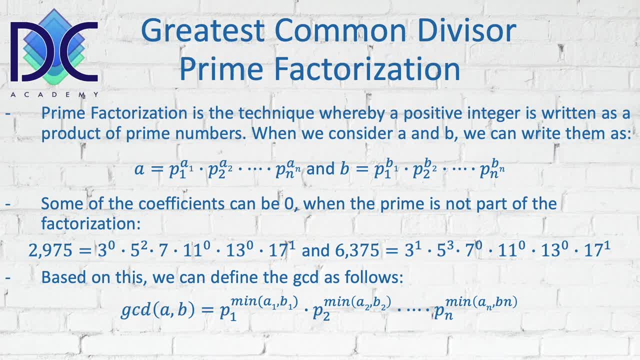 So I have P1, I find it in A and in B and I use the power which is the minimum of the power of P1 for A- A1, or the power of P1 for B- B1. And I do that for all the relevant powers that I have. 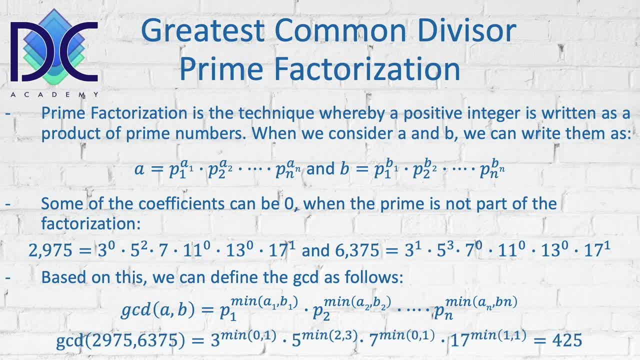 It will be better if I show you on the example we have above. So when we have the greatest common divisor, we can say that The greatest common divisor between 2,975 and 6,375 is three to the power, the minimum of the powers of three, which are for A, zero and for B, one, multiplied by five, to the power, the minimum of two and three. 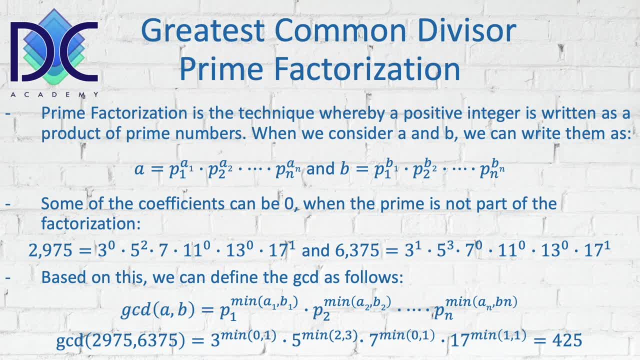 So in 2,975, we have five to the power two, And in 6,375, we have five, We have the next one, which is seven. We take the minimum between zero and one, and then we take 17,, and the minimum there is between one and one. 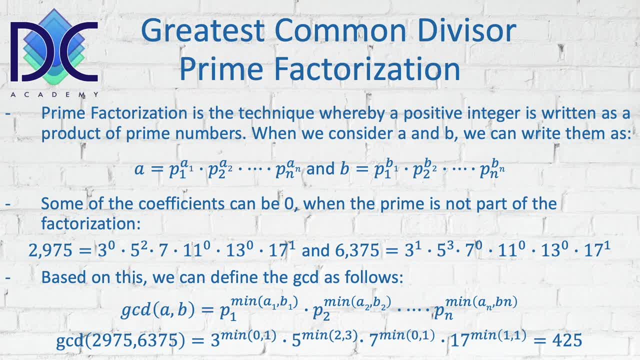 So I took out 11 and 13,, because both of them have no power, let's say are not part of the factoring of any of those numbers. So I have to take three. The minimum zero of one is zero, So it becomes three to the power of zero. 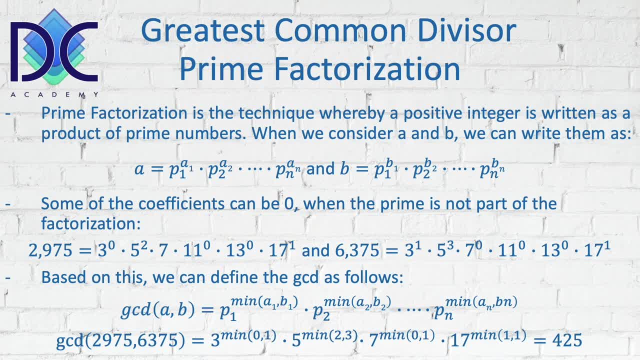 Five and to the power. minimum of two and three is then five to the power of two. Seven minimum of zero in one is also seven to the power of zero And for 17, I have the minimum of one and one. So we take 17 to the first power. 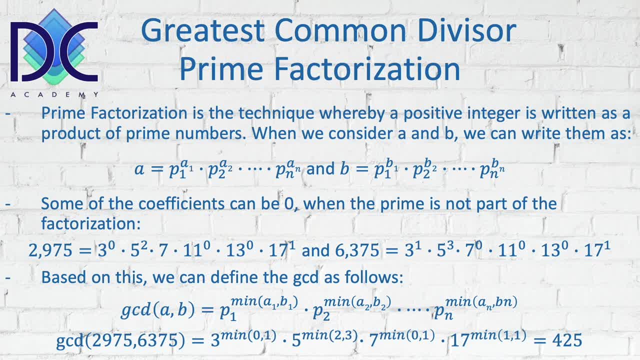 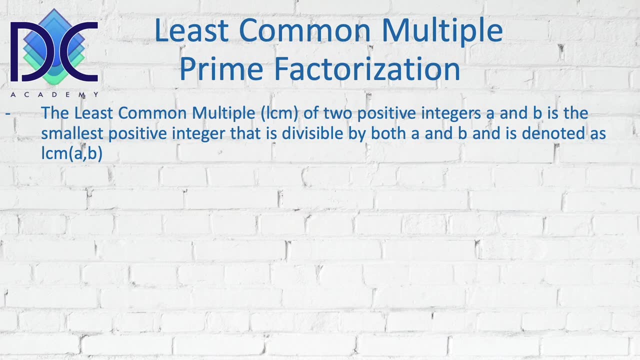 And when I look at this, we find that the greatest common divisor is basically 425.. Now we can also find, let's say, the least common multiple. And the least common multiple of two positive integers, A and B, is the smallest positive integer that is divisible by both A and B. 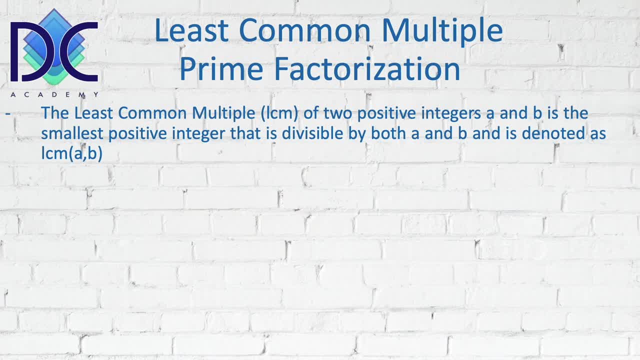 And we write it as the least common multiple of A and B. LCM is the abbreviation. So based on the prime factorization, we can say that the LCM is of two numbers: A and B is in fact, when we look at their prime factorization.